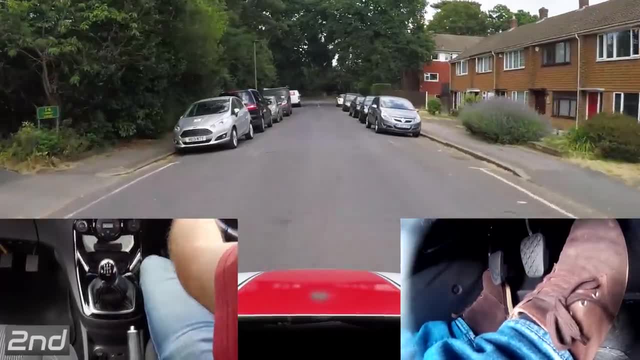 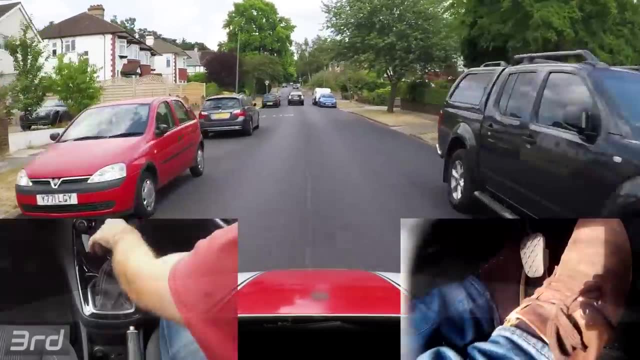 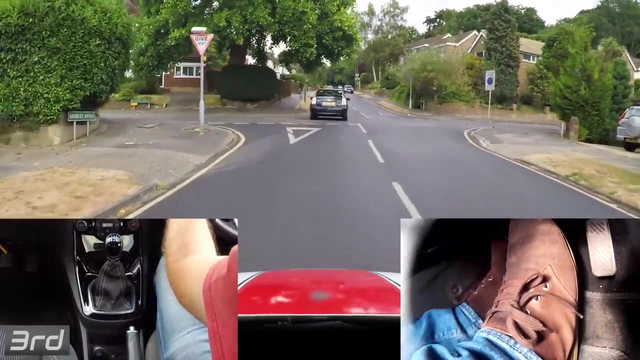 If you're not confident doing this, then just use the parking brake, as it's so much easier. Let's try another junction. When moving off uphill, you've got to make sure that you press the gas pedal or there's a good chance the car will stall. You must also find the biting point. 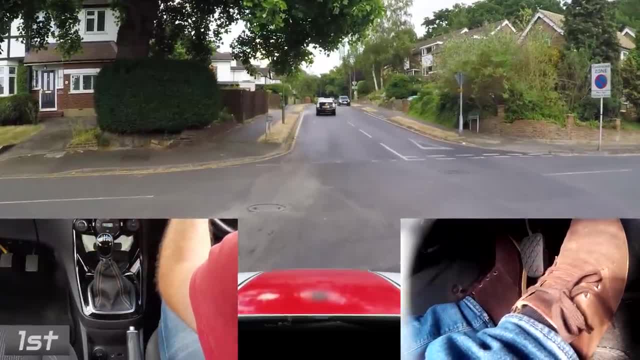 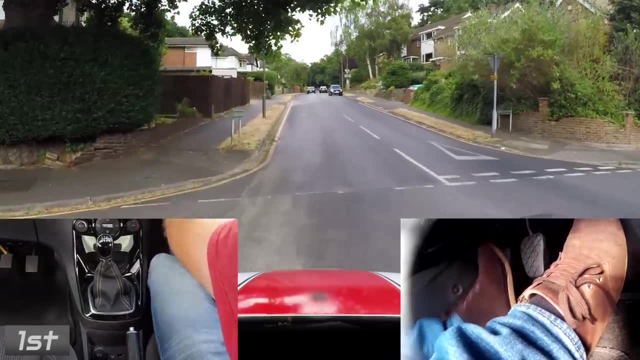 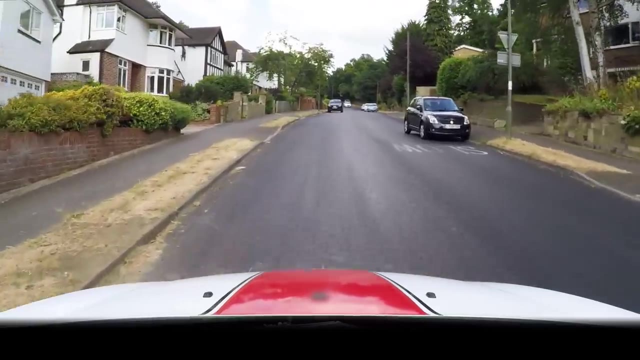 quickly or the car might roll back. but you could also stall. if you release the clutch too high, Then slowly release it. If the car moves off too fast you can always lower the clutch to slow down- roughly- the thickness of a pound coin- or raise it a little to move more. 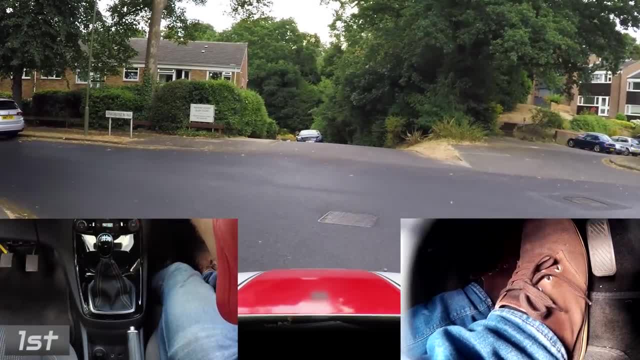 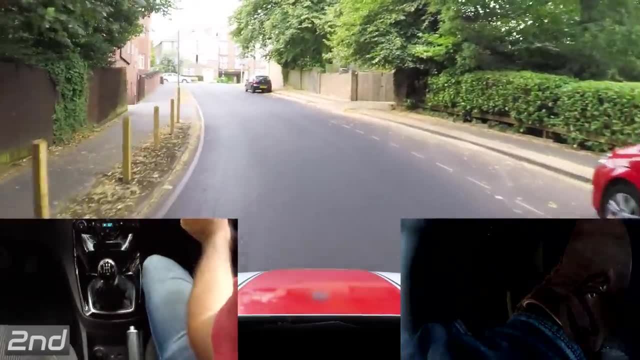 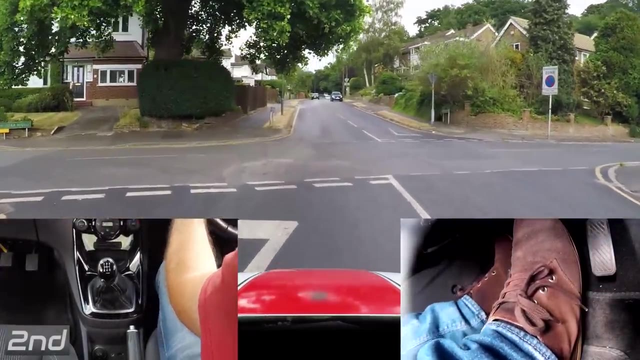 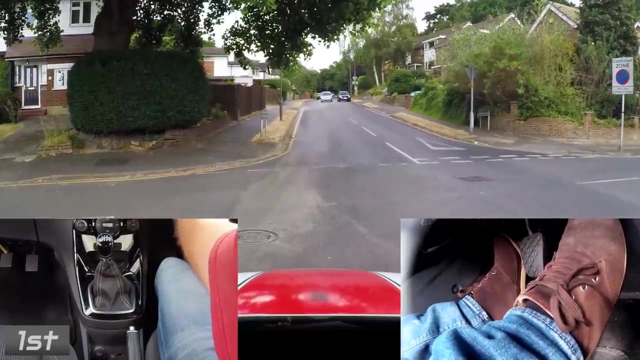 As always, I'd highly recommend practicing with an instructor, somewhere quiet to start with. Don't forget: if you're not confident doing hill starts this way, then just use a parking brake. Let's do another one. Off the brake. gas biting point: feet steady for a couple of seconds. 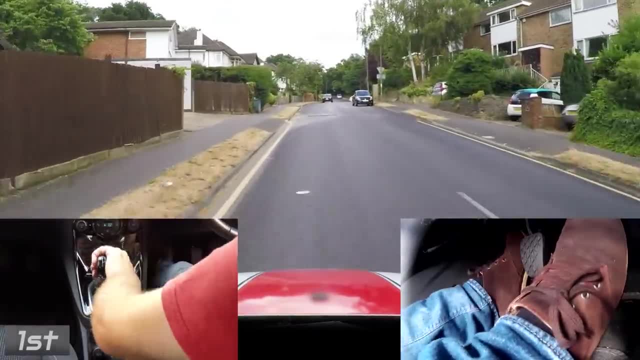 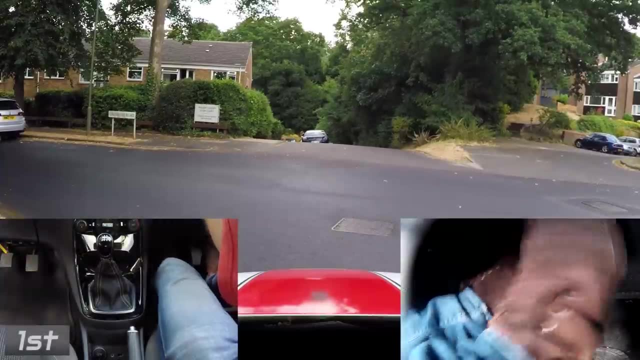 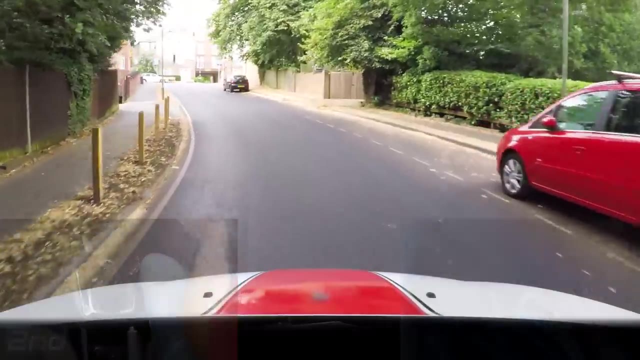 more gas as a clutch slowly comes up. You certainly need to be fast with your feet, but in control. You don't want the car to roll back, zoom off or stall. Let's do one more And then away we go. Now we'll show you a different way of tackling these junctions. 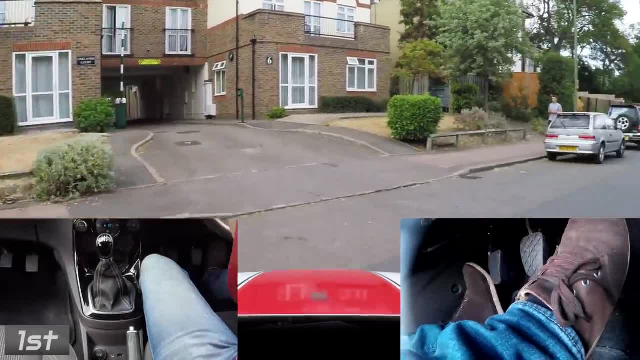 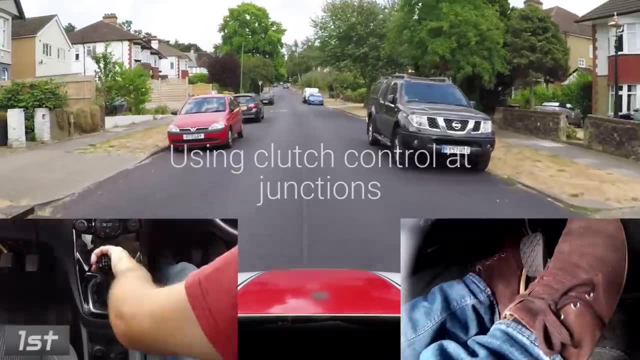 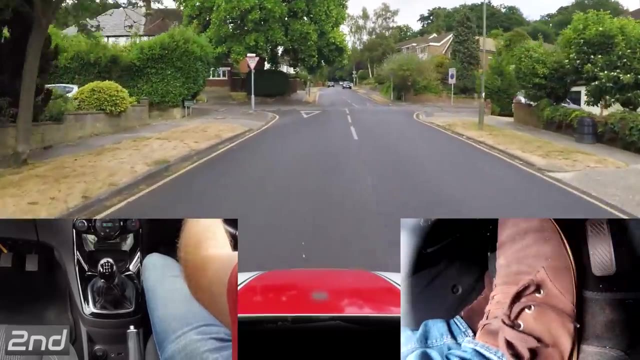 Don't forget to press the gas pedal and then hold the biting point for a couple of seconds to avoid stalling. I'm heading back to the same junctions again and this time, if it's definitely clear and safe, I'm not going to stop, as there's a giveaway line and not a stop line. 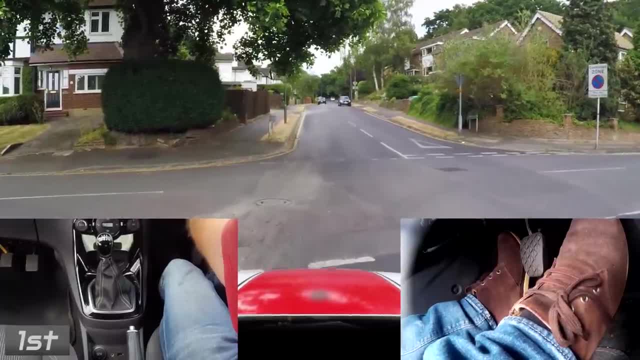 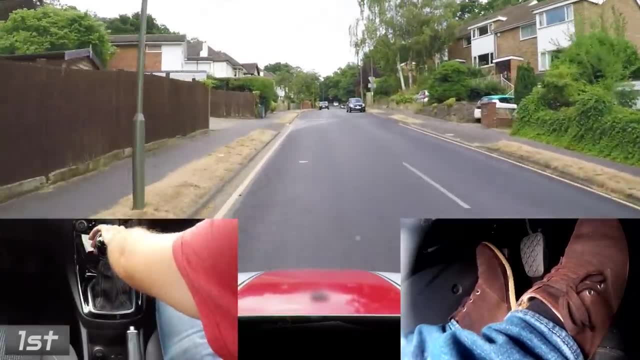 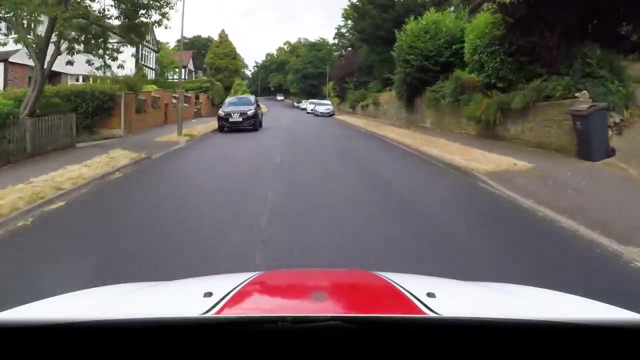 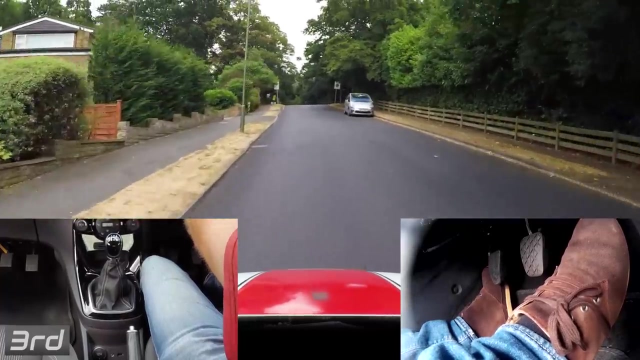 It's tricky to see. so I need to creep out really slowly using some clutch control, Observe properly and be ready to stop Another junction and again I've got to give way. As long as it's definitely clear and safe, I don't have to stop, but always ready to. 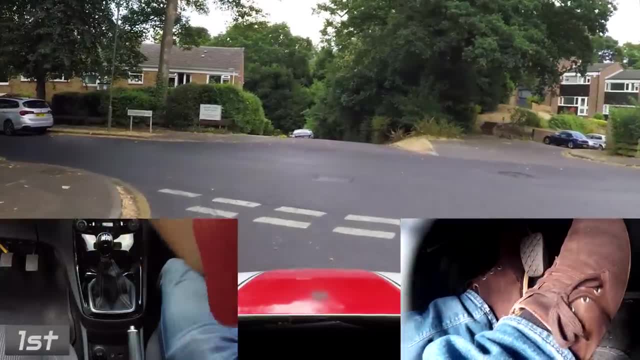 Clutch down first gear. set the gas biting point feet. steady. Clutch down a little more and we're ready to go. Clutch down first gear. set the gas biting point feet. steady. Clutch down a little more and we're ready to go.